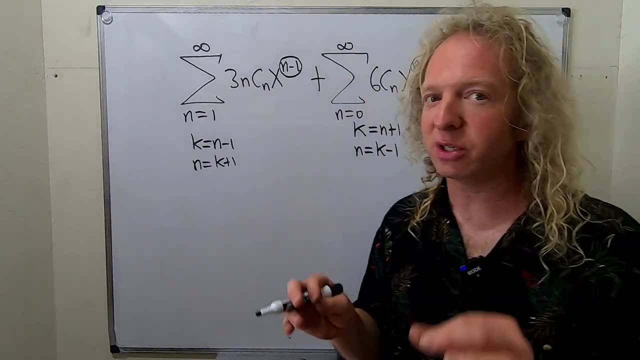 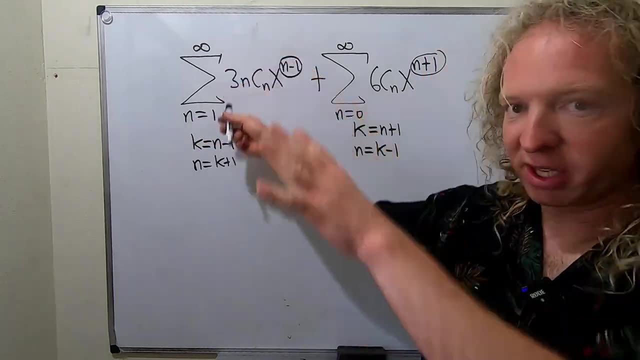 of the summation. This is a super important technique. You can do it in your head. Some people do it in their head. I like to show the work. Okay, so now we're going to go ahead and replace the sum with whatever we end up with. So again, you call it k. solve for n. Call it k. 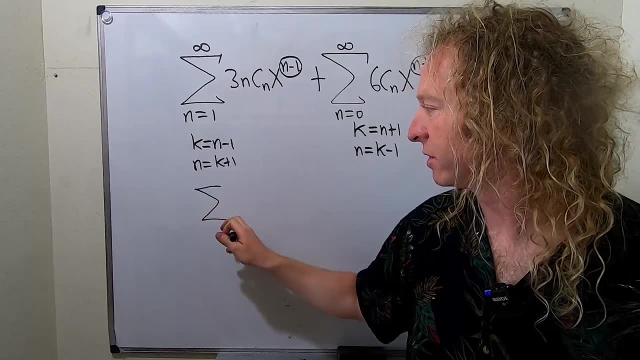 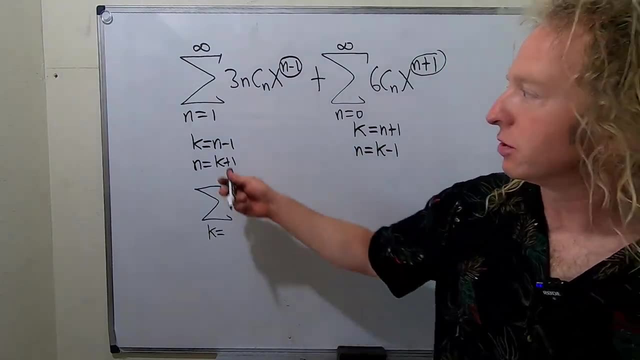 solve for n Good stuff. Let's rewrite our sum. So we have the sum Now. everything is k, So it's k equals. Okay, let's see where we start. So if n is 1, you can take the 1 and plug it in here. So k is 1. 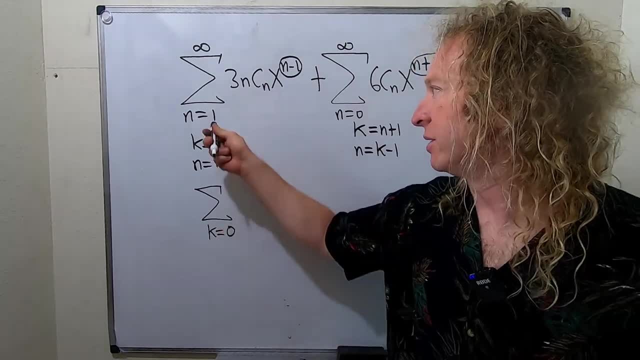 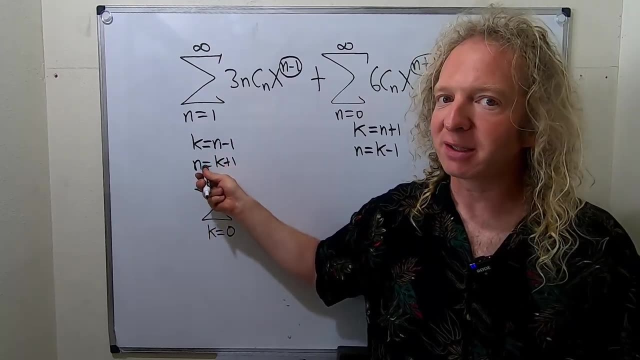 minus 1, which is 0.. Again, just take this and put it here: 1 minus 1 is 0.. We're still going to infinity. Now we're going to use the fact that n is k plus 1.. So it's 3k plus 1.. So 3 parentheses. 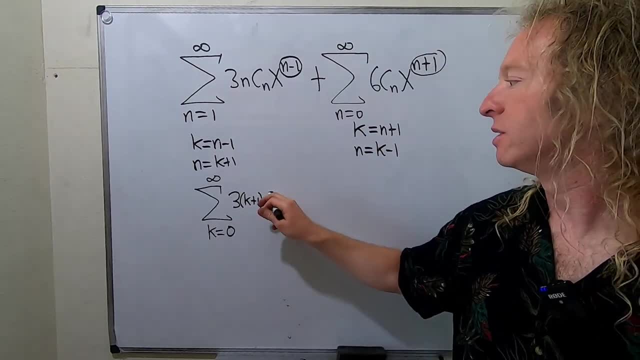 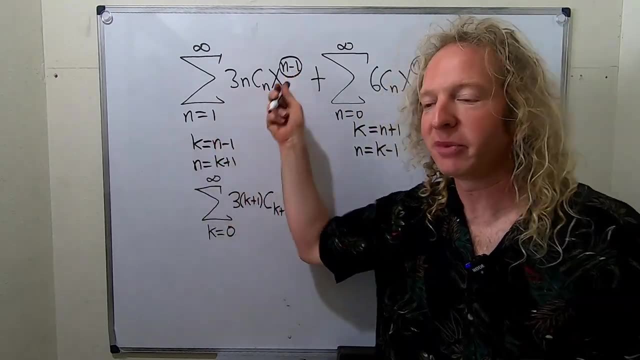 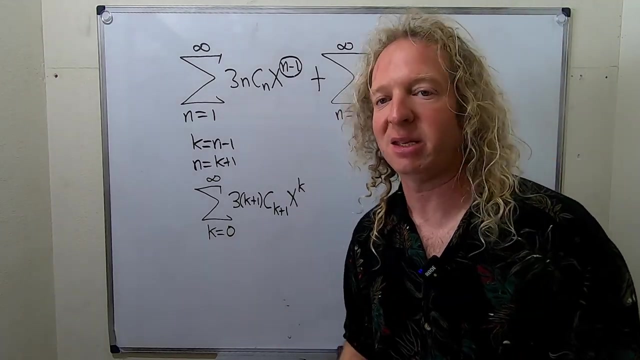 k plus 1.. Really delicate stuff: C sub k plus 1.. x to the k. That was the whole point. I always tell myself: that is the whole point. The whole point is to make this a k. We want them all to be k's. Let's go to the next one Plus All right. 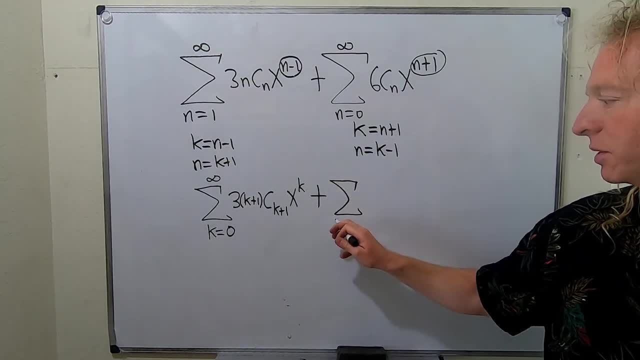 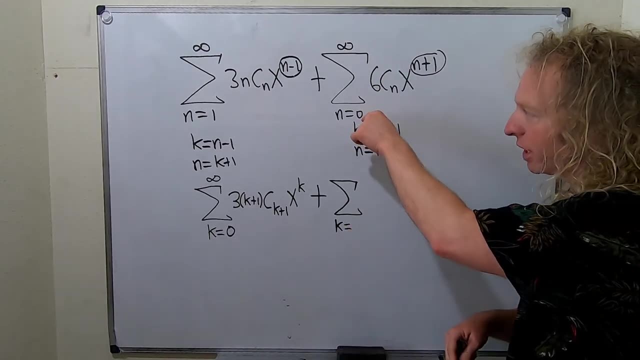 let's see what's happening here. So we have the infinite sum, And we know it's going to be k equals. And now we're going to do the same thing. We're going to figure out where to start this infinite sum. So when n is 0, k is 0 plus 1.. So we're going to do the same thing. We're going to 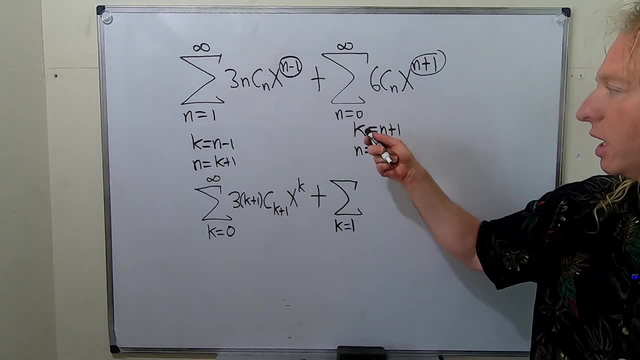 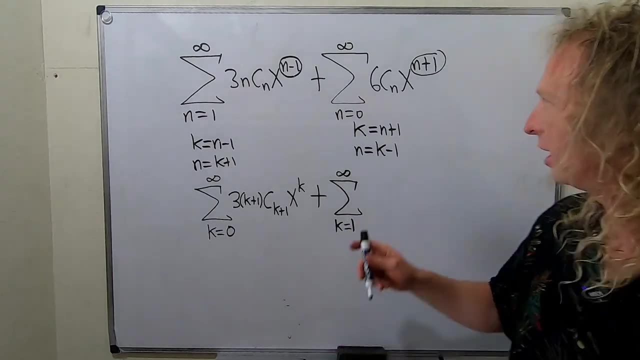 do the same thing. So k is 1.. Again, when n is 0, you get k equals 0 plus 1. So you get 1. And we're going to infinity. Really, really powerful technique. Then we still have the 6. And n is k. 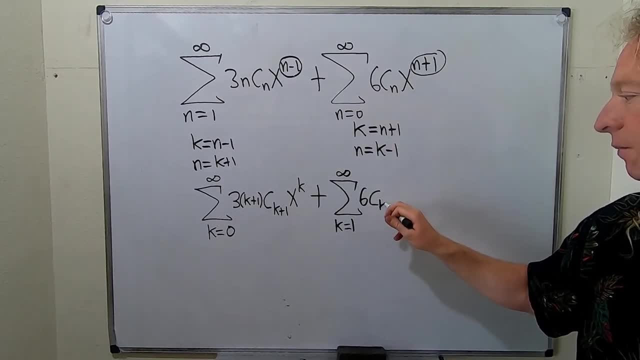 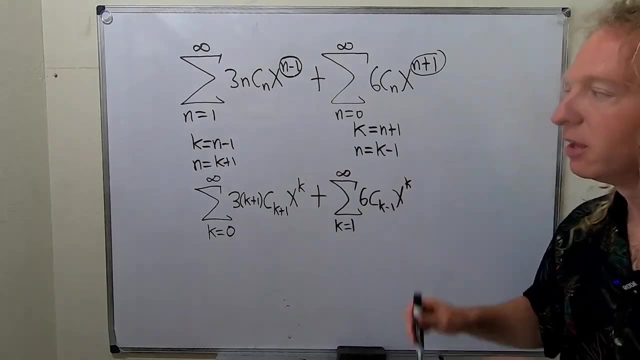 minus 1.. So we get c sub k minus 1.. And then x to the- oh wait, that's k, And that's the whole point. The whole point is to make these x to the k's. So recap: Call it k, solve for n. call it k. 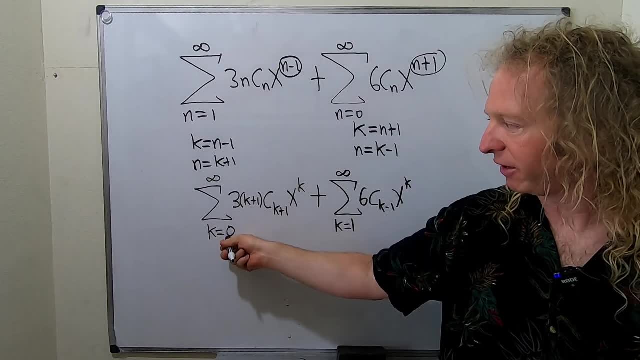 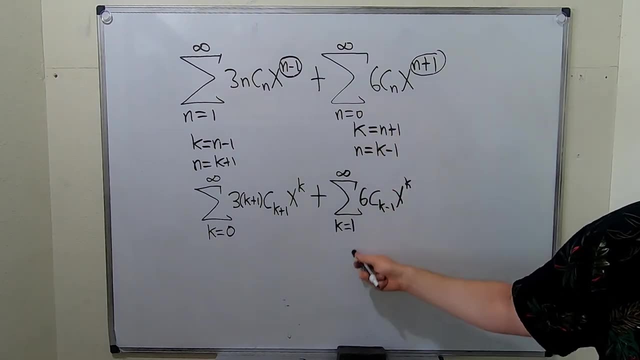 solve for n Everything very carefully Again. to figure this out, you just take this number and plug it in: 1 minus 1 is 0.. To figure this out, you take this number and plug it in: 0 plus 1 is 1.. 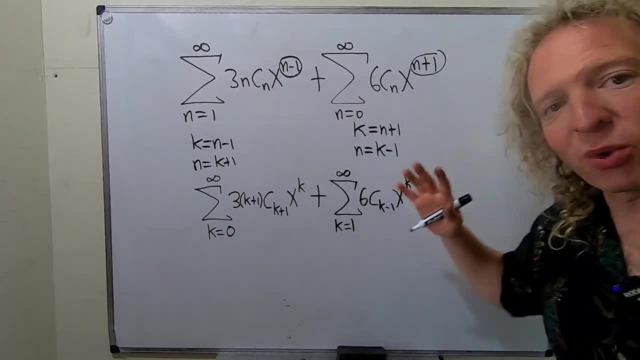 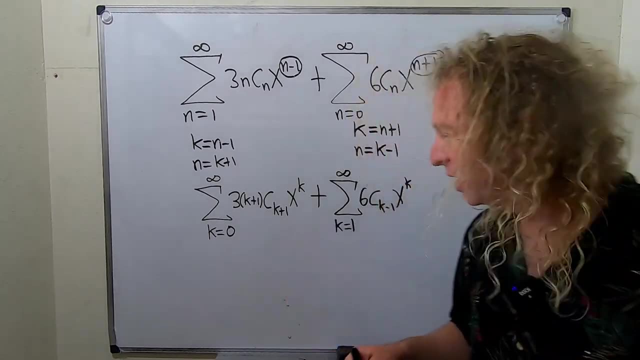 OK, this next step is a little bit tricky, So we want to write this as a single sum. So you always want the easy way to do it. There's a bunch of ways to do it, But the easiest way, in my view, is to start at the highest 1.. So we have 0 and we have 1.. So we want them to start. 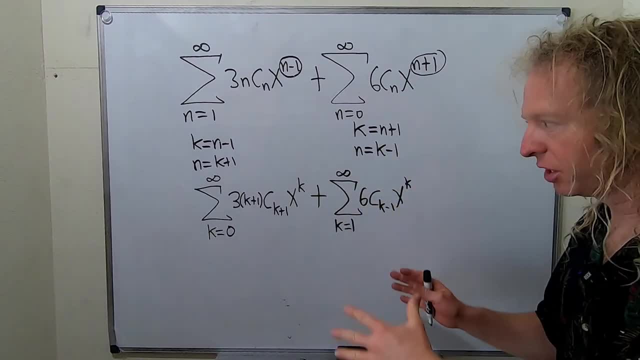 at 1.. So you want both sums to start at 1.. So here's what you do: You start this at 1.. You might say what You can't do, that Yes, we can. We will make it right. 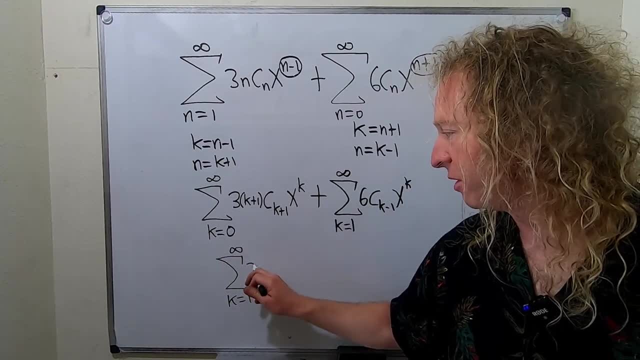 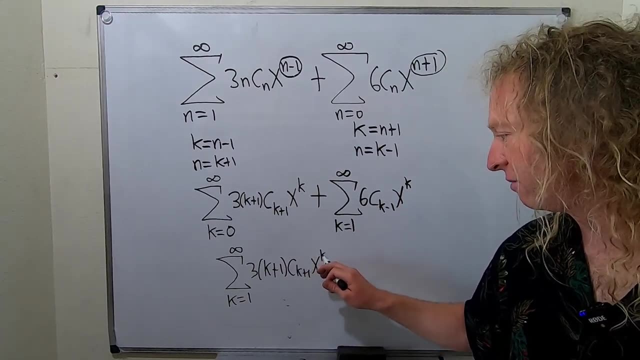 Watch this. I'm going to write it all over again. I'm going to start at 1.. So we have 3, k plus 1, c sub k plus 1, x to the k. So I started at 1, which technically is still wrong plus. 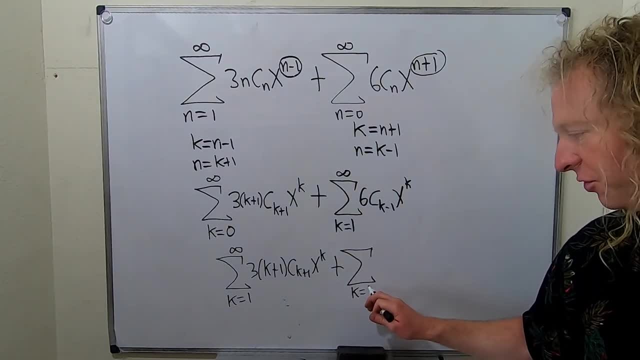 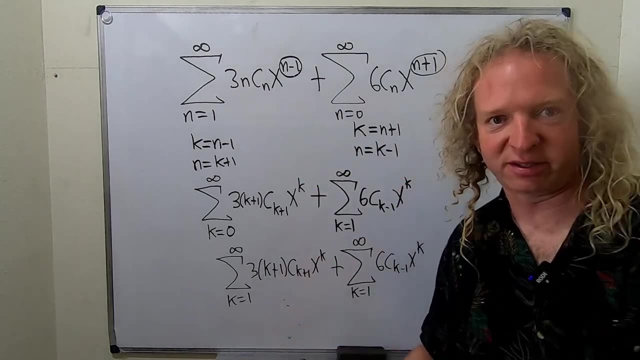 But we're going to fix it. k equals 1 to infinity 6, c sub k minus 1.. I love these problems, So this is not equal to this. At this point, this is incorrect. These are obviously not the same. This is this. 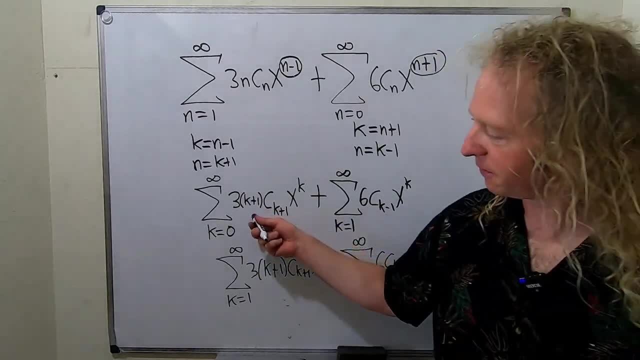 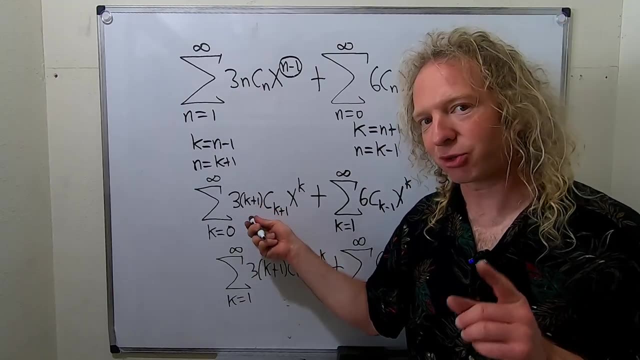 but this is not this. So let's think about this. What is this? This is the sum from 0 to infinity. This is the sum from 1 to infinity. This has an extra term. It has the 0-th term, So we're missing. 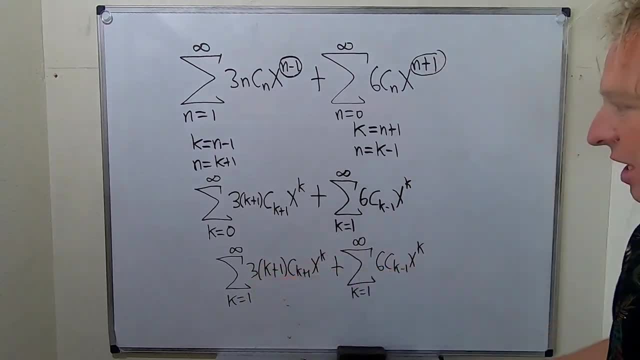 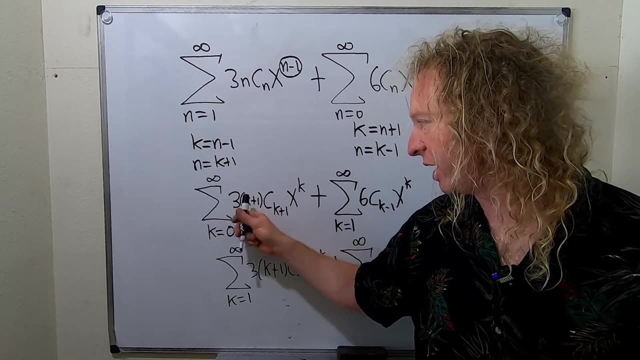 that 0-th term here. So what do we do? We have to write it down. So how do we do that? We just plug in 0. So if you plug in 0 here, you get 3 times 0 plus 1. So you get 3.. 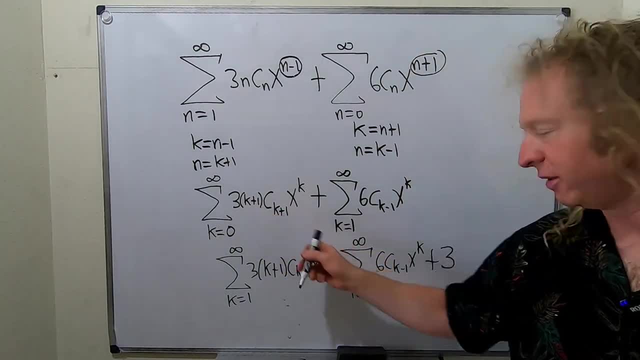 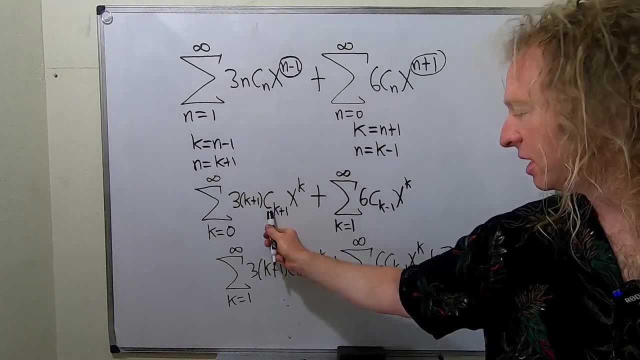 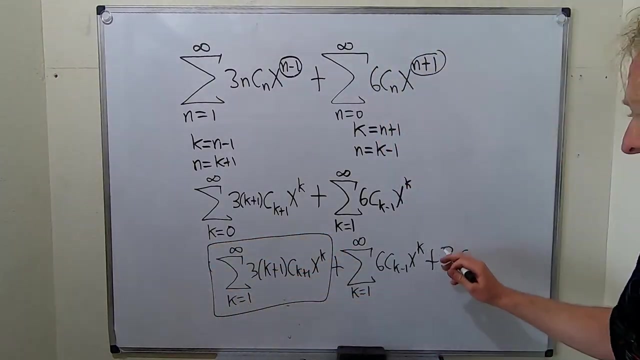 c sub 1, x to the 0 is 1.. Again, if you plug in 0 here, you get 3.. c sub 1, x to the 0 is 1.. So now what's happened is that this, together with this, is equal to this right: These two. 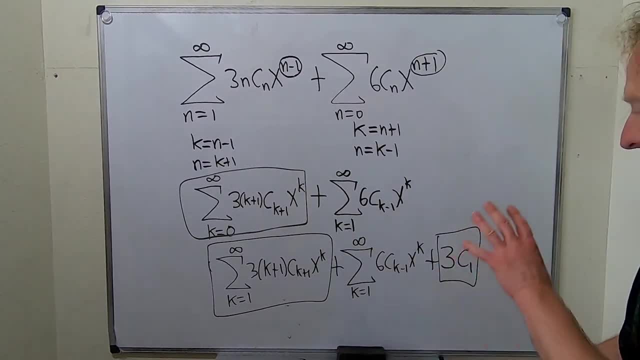 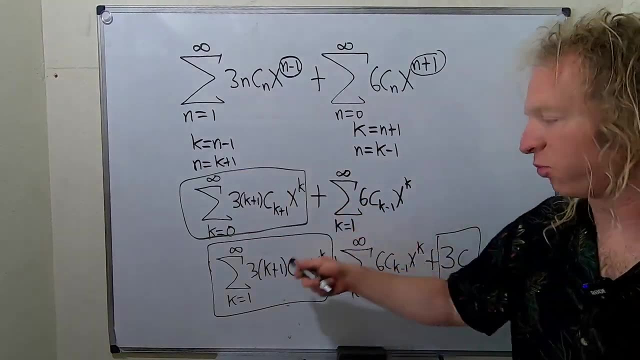 are the same as this, because this is the sum from 0.. This is the 0-th term and this is the rest of them. So this is all of them. 0 to infinity. this is 0, and then it's 1 to infinity. So 0 to infinity is the same thing as.